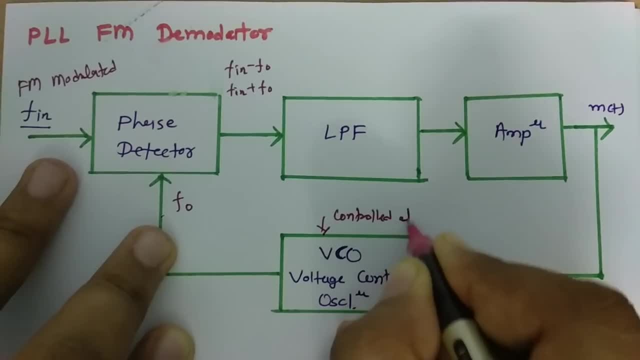 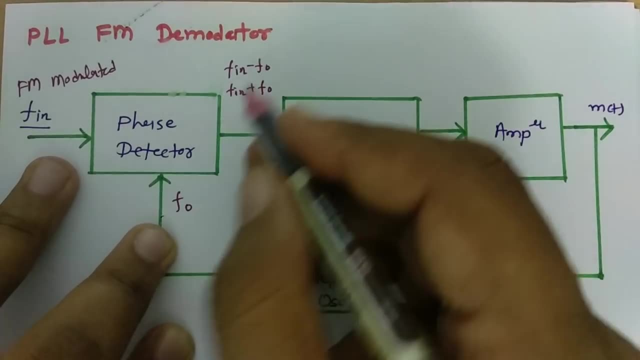 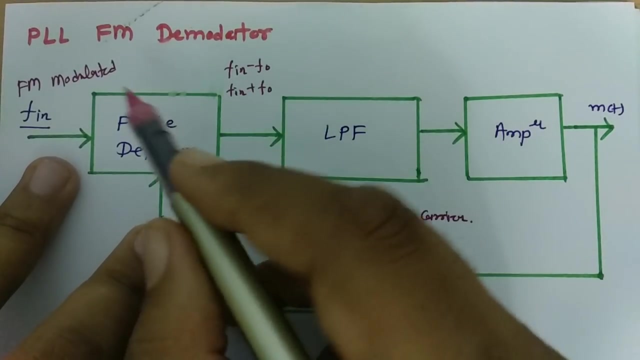 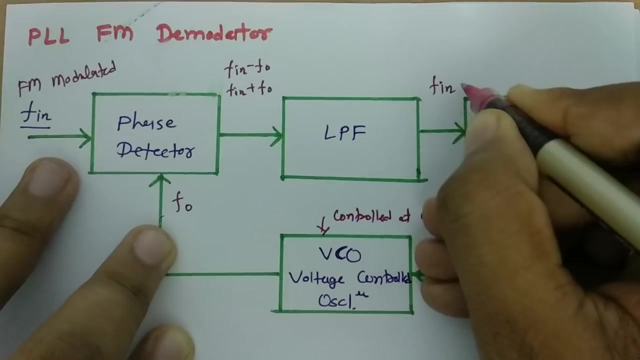 So the there is to modulating signal is controlled. So as this VCO is controlled at carrier, this, this two frequency component, where lower frequency component will be having information that is related modulating signal. So when you pass this signal through low pass filter you will be getting FIN minus F0 frequency component over here and when. 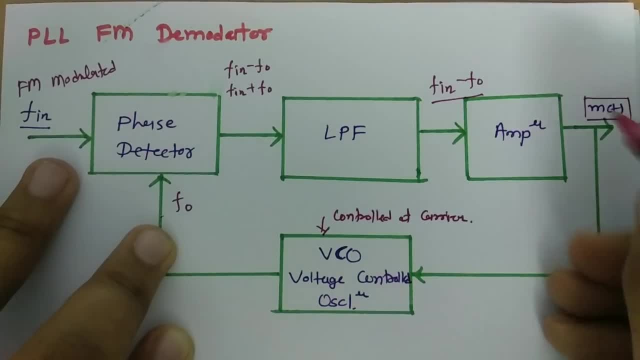 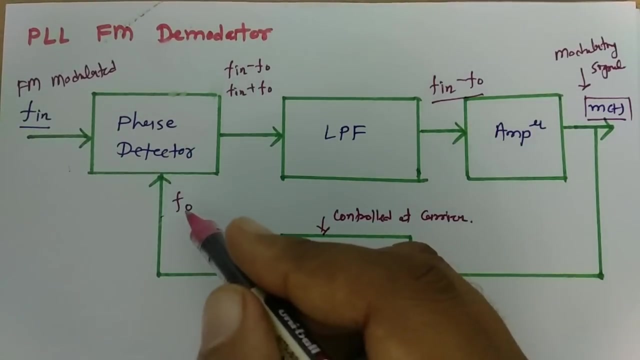 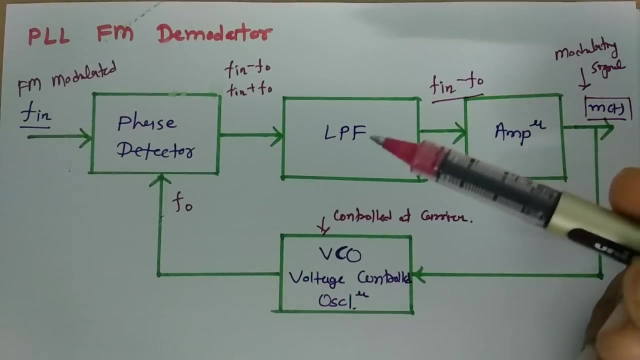 you amplify that, that will be resulting into modulating signal. So this is how we do: demodulation, like see VCO, that is controlled at carrier, that generated frequency is actually given to phase detector. Output of phase detector is equals to the frequency output of phase detector. that will 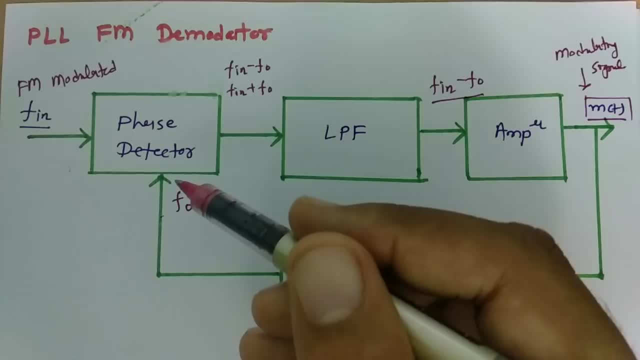 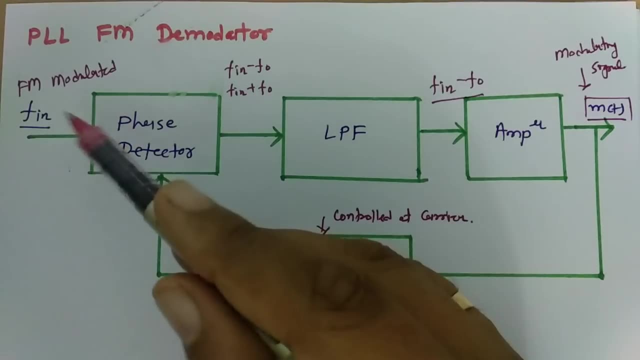 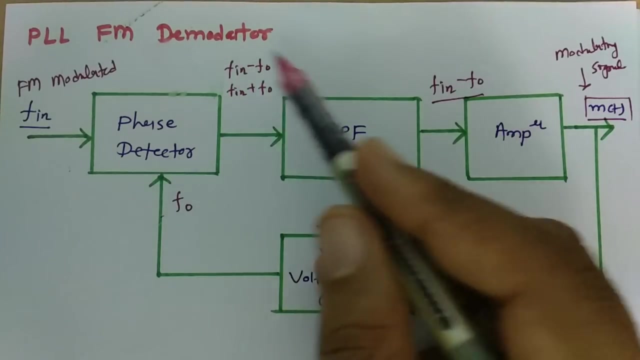 be similar to that multiplier, So it will be generating two components. one is f in minus f0 and second is f in plus f0, and when you pass it through low pass filter you will be getting lower component of frequency, that is, having modulating signal, which is what f in minus f0. 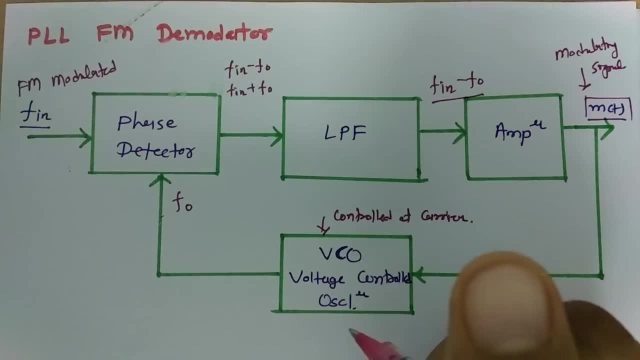 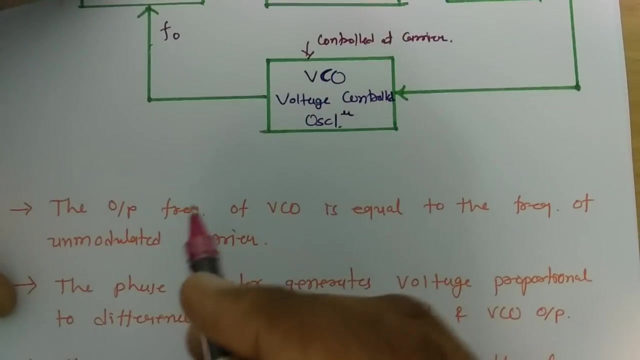 So at output of low pass filter you will be getting f in minus f0.. And here, if you see the basic understanding, then this VCO that is controlled at carrier signals frequency. So let us see what are the basics which is there with this output of output frequency. 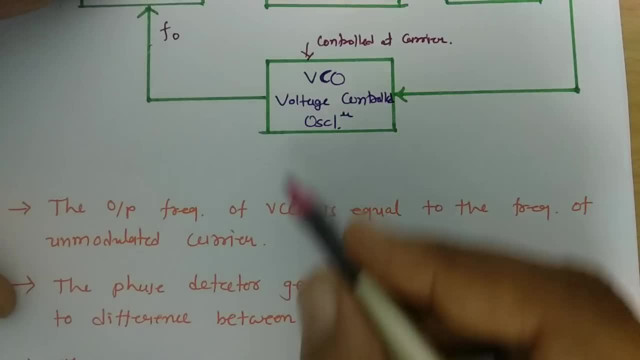 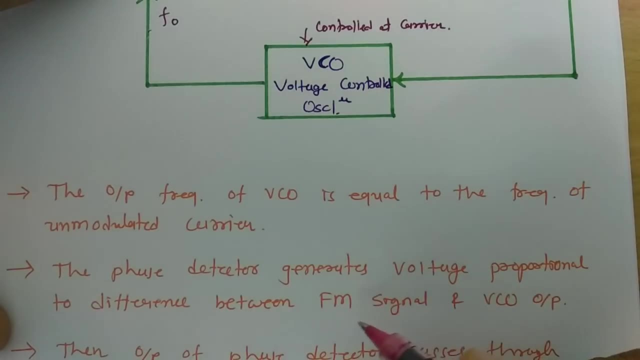 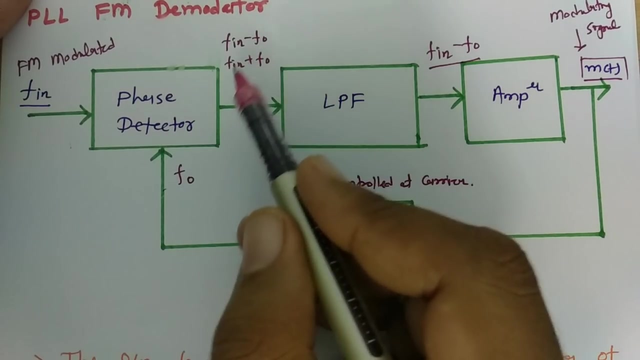 of VCO is equal to frequency of unmodulated carrier, So it is focused at carrier. The phase detector generates voltage proportional to difference in between FM signal and VCO output. So it is actually giving two components: f in minus f0 and f in plus f0. 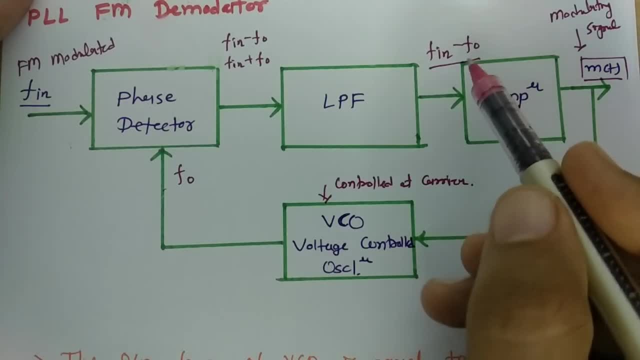 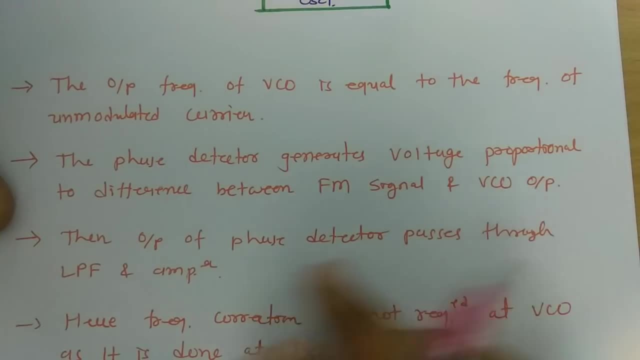 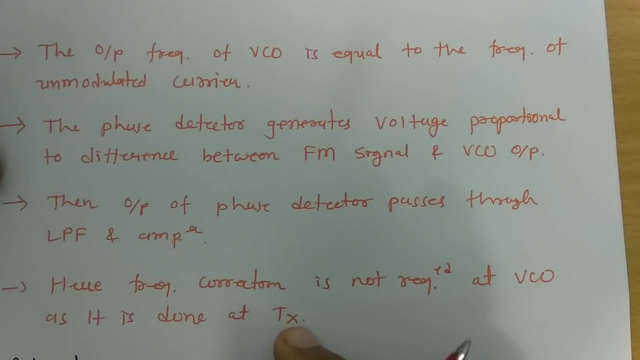 But after passing through low pass filter you will be getting f in minus f0. So we are focusing on that difference. Then the output of phase detector passes through low pass filter and amplifier. Here frequency correction is not required at VCO as it is done at transmitter section.